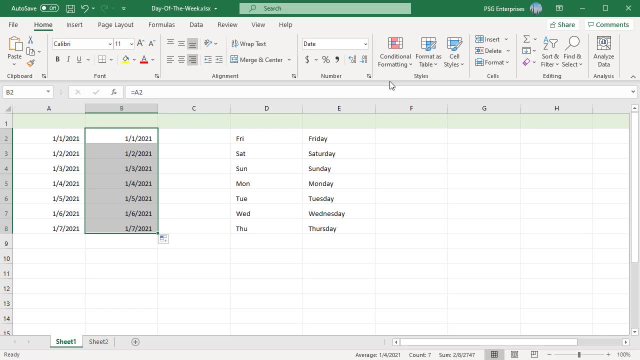 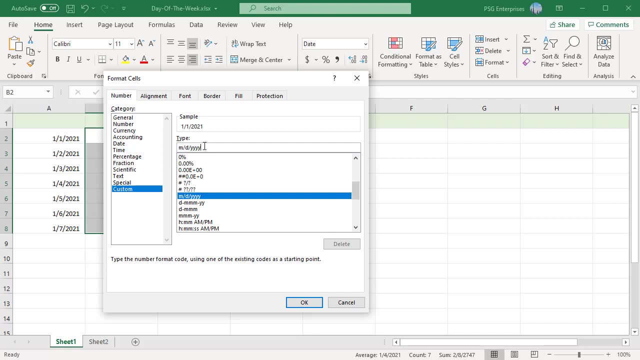 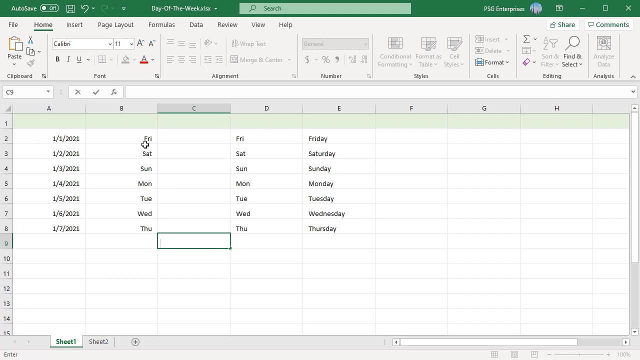 Open the format cells dialog box. Click on custom. In the type text box, enter 3Ds to display an abbreviated day name. The sample box displays how the output is displayed. Click on OK. Days are displayed as FRI for Friday, SAT for Saturday, etc. 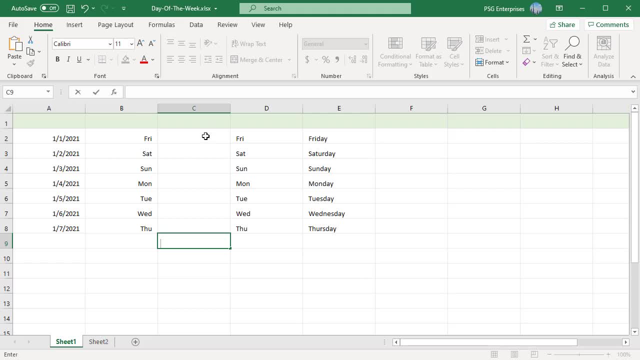 To display full day names. In the type text box, enter 3Ds to display an abbreviated day name. In the type text box, enter 4Ds to display an abbreviated day name. Day names are displayed as Sunday, Monday, etc. 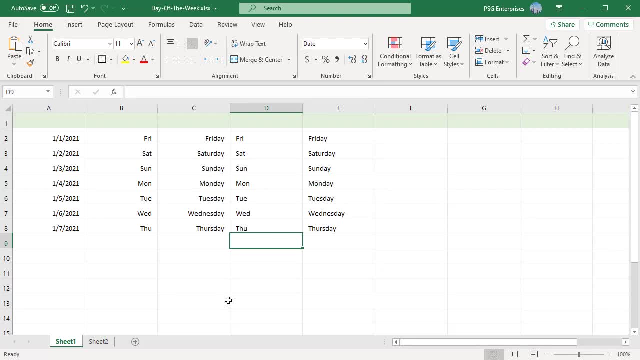 The values in the cells are still dates which can be used in calculations Only. the format is set to display only day names. As dates are aligned to the right by default, You can see that these values are aligned to the right. You can use the text function to display the day of the date. 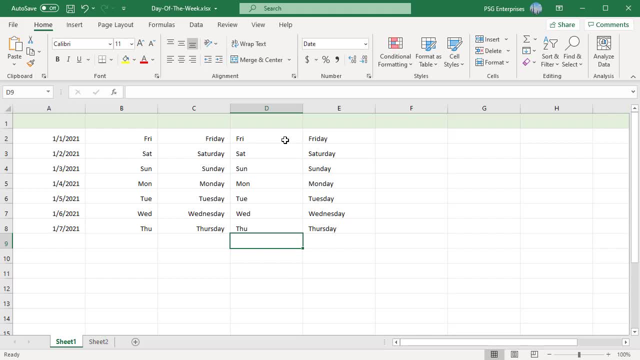 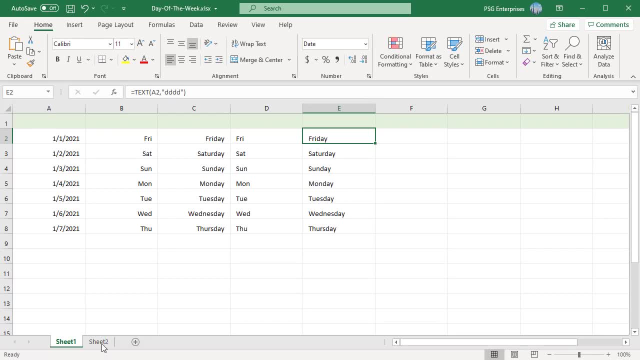 You can also use the choose and weekday to return a custom day name. You can also use the choose and weekday to return a custom day name. You can also use the choose and weekday to return a custom day name. custom day name- Weekday function gets the day of week as a serial number One for Sunday. 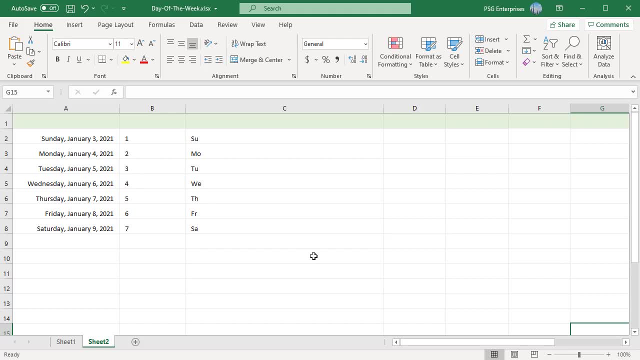 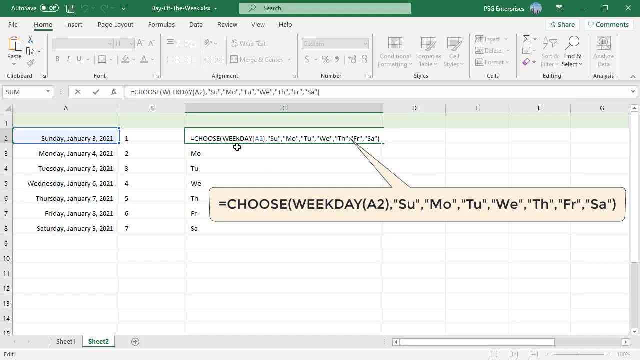 two for Tuesday, and so on. Choose selects a value based on index number. Use this formula. The choose function uses the return value from weekday as index num. the first argument That indicates which value from the list of value arguments to return Enter the weekday. 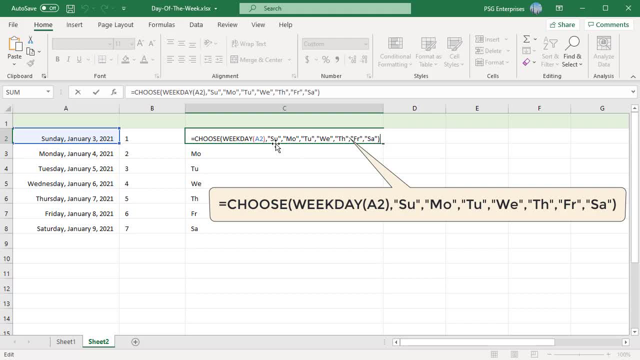 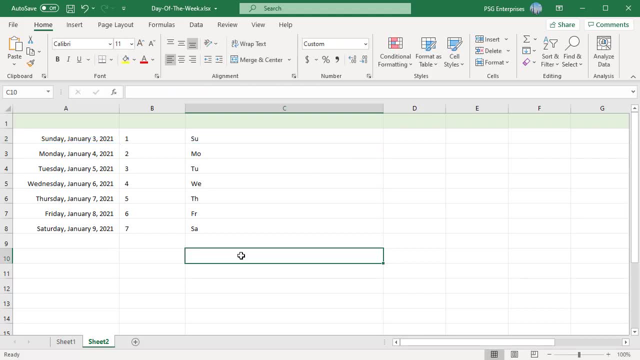 names you want to display as the value arguments. For example, if you want two letter weekdays, enter SU for Sunday, MO for Monday, etc. To download example excel file, please click on the link in the description. If you like this video, please subscribe to our channel.